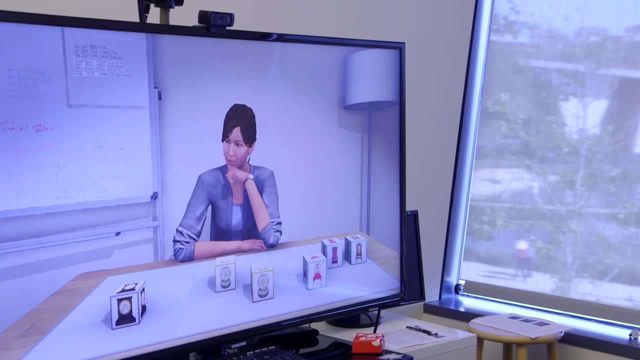 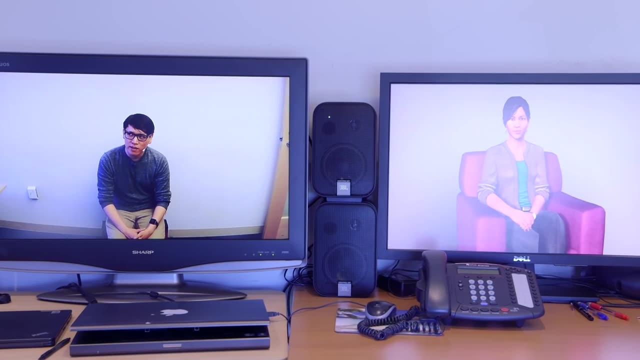 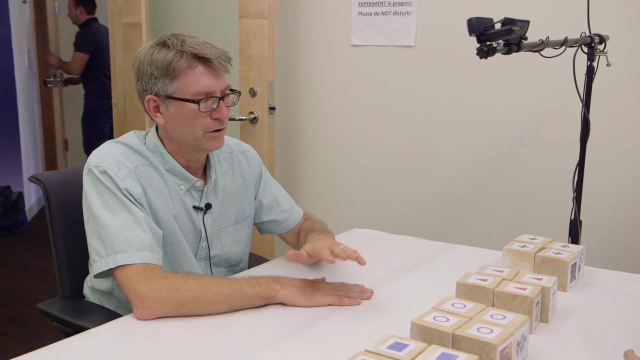 Sounds great. How do you think we should split up the items? All of these intuitive behavioral norms we learn at a young age- Okay, We learn at a young age- are actually really difficult to program into AI. Currently, the negotiation agent can say 5,000 things, and those all are verbatim things that the humans we brought in said in their negotiations. 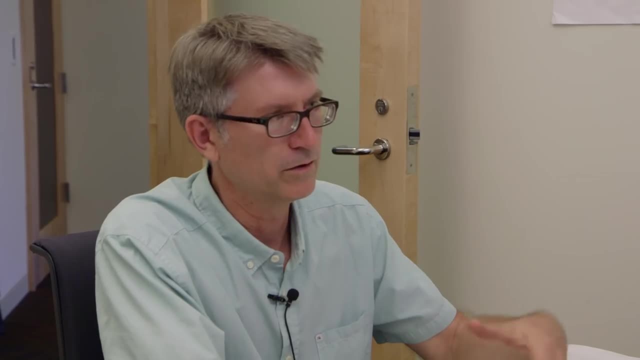 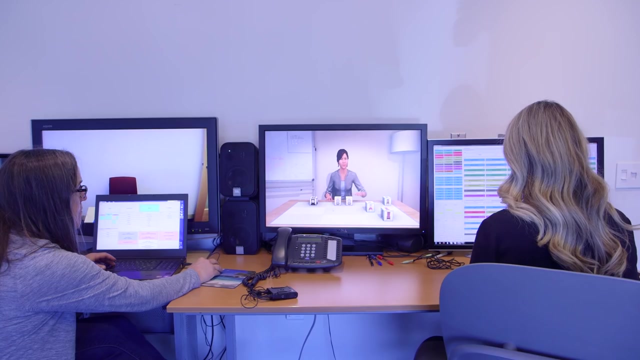 And this negotiation agent that you interacted with. she's still controlled by a wizard, In fact two wizards: One is doing the decisions and one is doing the nonverbal communication. Okay, So what we've done here will have implications far beyond the therapist's office and even business schools. 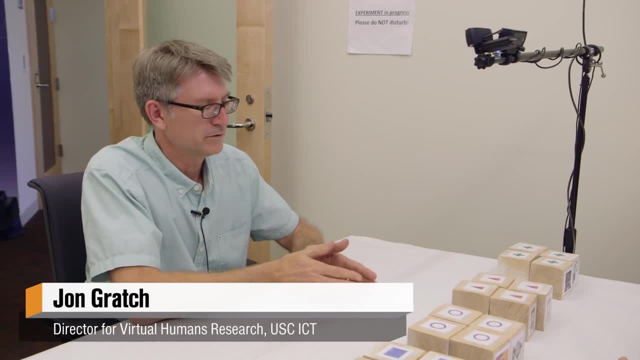 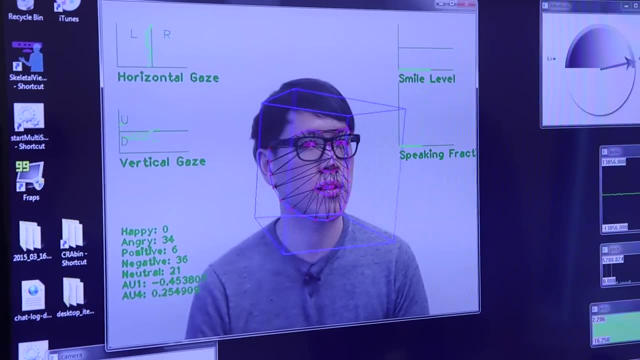 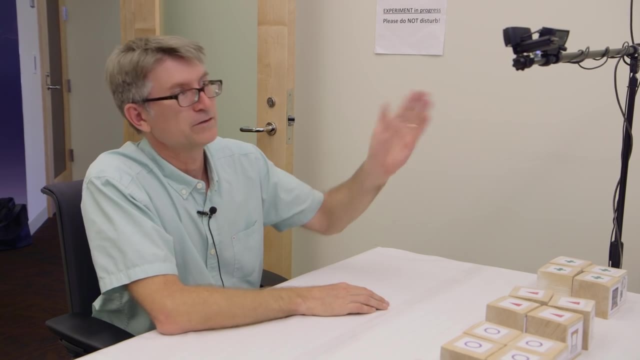 As John Gratch, director of the virtual humans research at USCICT, explained to me, the AI of autonomous cars, for example, will need the ability to operate in the social environment of city street traffic. So when I'm crossing the street in LA, I look to that car and I look to that driver and I see: does that driver see me before I cross the street? 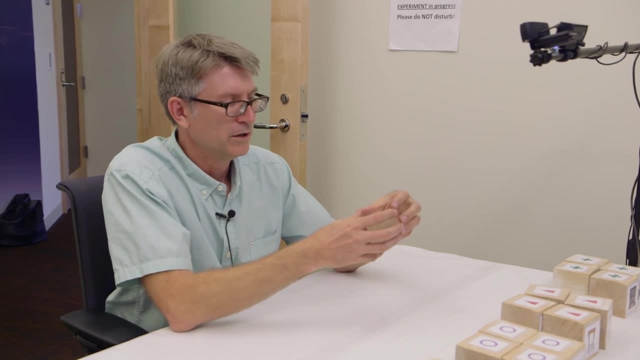 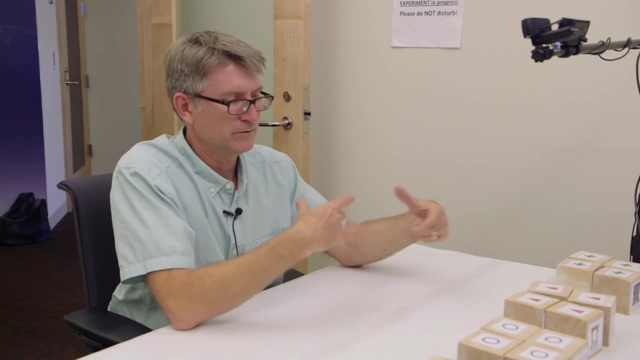 That's a sort of social intelligence, Okay, And when I make a mistake I say oh, I'm sorry, I'll do better next time. And those are things that I think fully autonomous systems will have to incorporate into their capabilities. 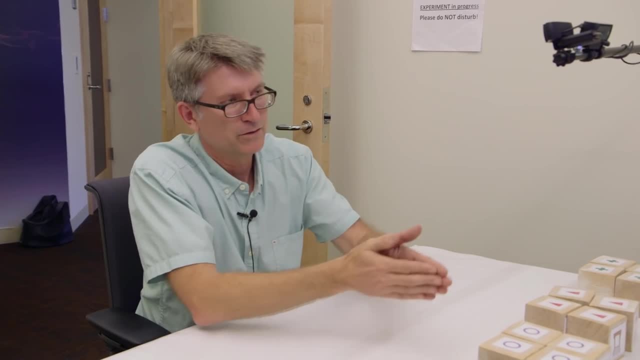 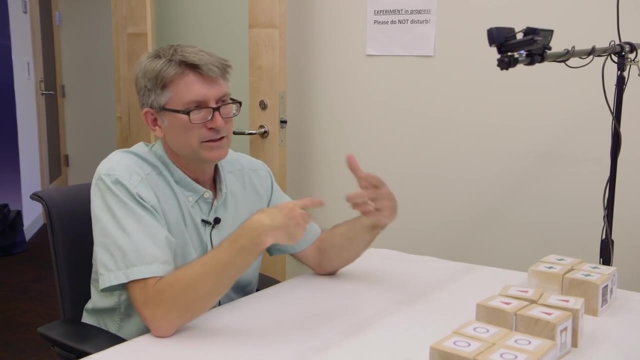 So when Google is going to navigate through New York City streets, it has to send signals somehow: Oh, I see you, I see you. Social niceties, politeness, all that kind of stuff actually serves functions and relationships. It makes communication more efficient. 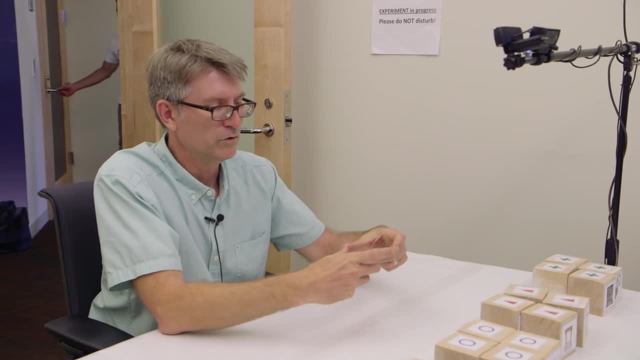 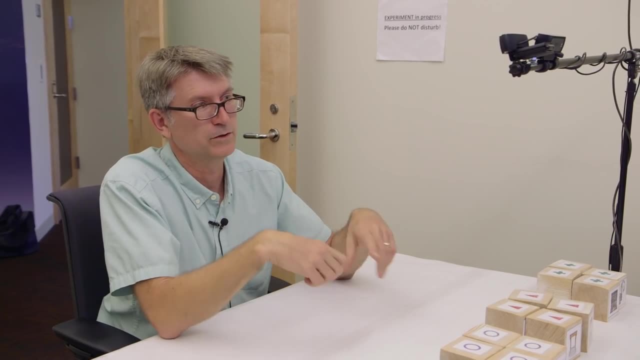 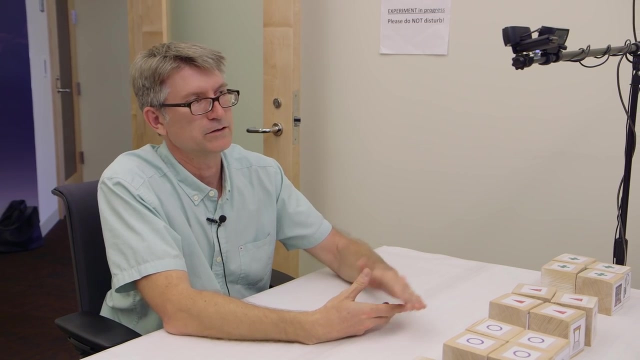 It tells me who I can trust. Okay, And as we move away from simple automation to autonomous systems, that has their own goals and maybe not exactly the same goal. as a human user, it becomes more and more important to understand this kind of way that humans deal with that, so that machines can do that as well. 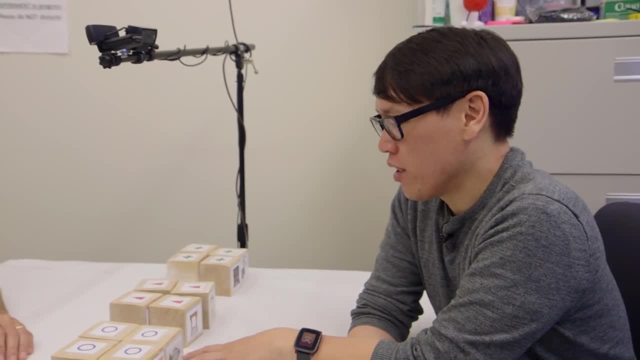 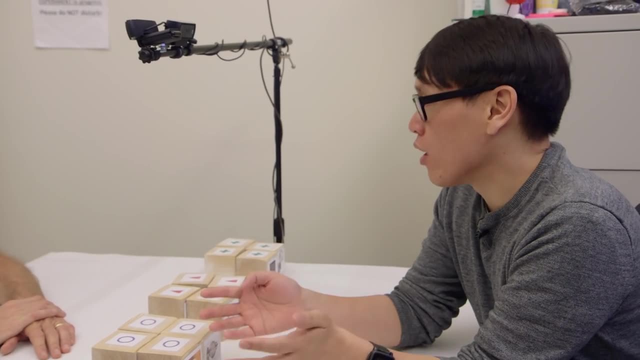 I mean those systems are coming. Yeah, I mean you look at the experiment like this and you can look at it and say, oh, you're trying to replace human-human interactions with human-computer interactions as a way to scale or to make it more accessible or for education.